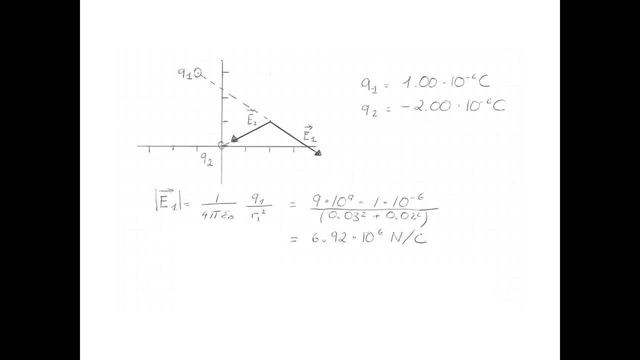 coulomb. The next thing to do is to figure out the direction of E1. So in order to help me with that, I'm going to redraw my diagram again. So I'm going to take the point in the fourth quadrant along the line that joins. 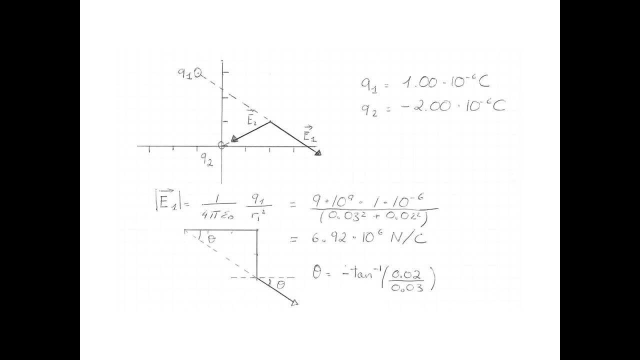 Q1 to the point where we're calculating the field. So that's three centimeters across and two centimeters down. So I take the inverse tan of the opposite side 0.02, over the adjacent side 0.03.. The negative angle just indicates that I'm counting the angle. 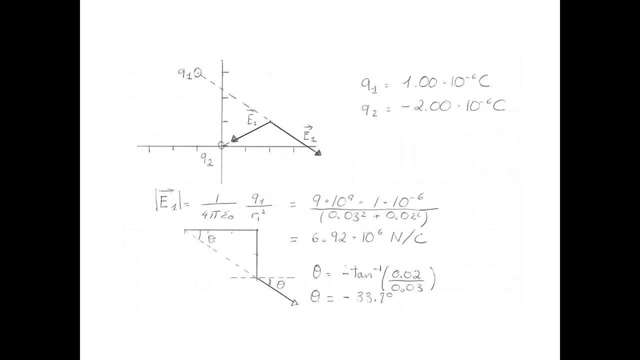 clockwise starting from the positive x-axis, That's negative 33.7 degrees. Next let's get the magnitude of our second electric field. Once again, using the formula for point charges, the magnitude of the second electric field is nine times ten to the nine. 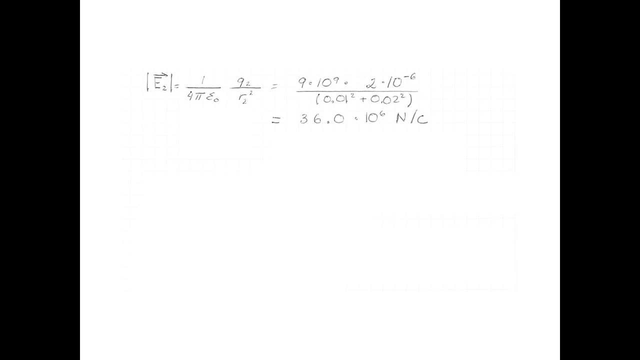 times two microcoulombs divided by 0.01 squared plus 0.02 squared, That makes the magnitude of the vector 36 times ten to the six newtons per coulomb. So I'm going to redraw a little sketch once again to figure out the direction. 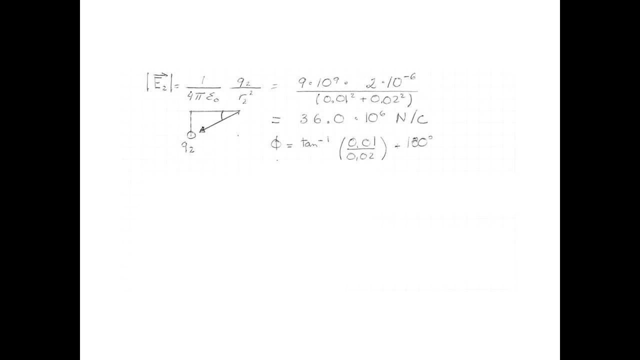 Here's a picture of the electric field vector pointing from P to the negative charge Q2.. The angle that I've drawn is the inverse tangent of 0.01 over 0.02.. But the angle of the vector is going to be that plus 180 degrees, because we're always counting from the positive x-axis. 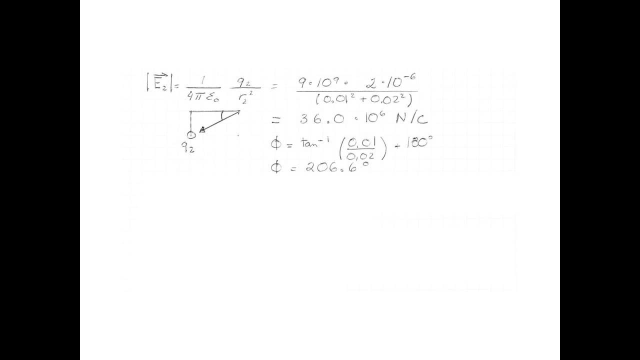 This makes the angle 206.6 degrees. Now we're ready to split up our two vectors into their components and to add them up. So in the x direction, we're going to add the x component of our first electric field, which is 6.92, 10 to the power of six cos. 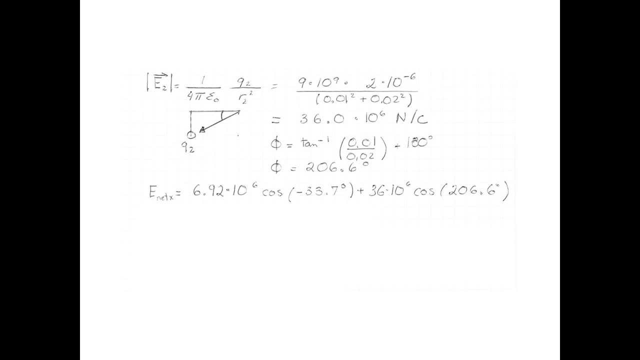 negative 33.7 degrees, and we're going to add the x component of our second electric field, So 36 times 10, to the sixth cos of 206.6.. I'm using cos in the two cases here because both my angles were defined from the positive x-axis. But if you would use some other convention, well, 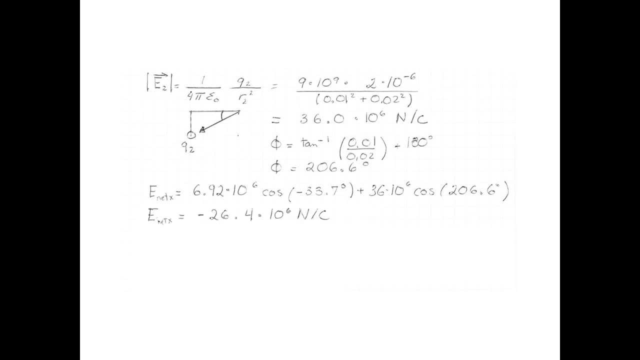 you might have ended up with a sine or even a tangent there. In the x direction our net electric field is negative 26.4 times 10 to the sixth newtons per coulomb. Let's add up the components in the y direction. The x component of E1 is 6.92, 10 to the power of six sine negative 33.7 degrees. 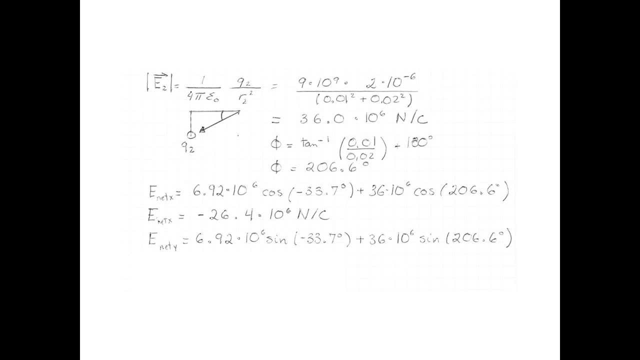 The y component of E2 is 36 times 10 to the sixth sine of 206.6 degrees. So the net field in the y direction is negative 20, 10 to the power of 6 newtons per coulomb. All right, let's get the. 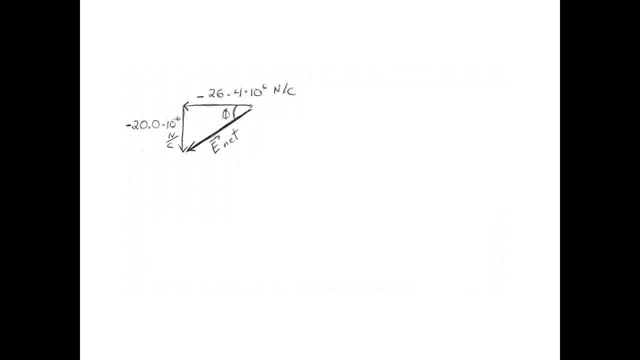 magnitude and the direction of the net field. Always, always, always, draw a picture of your new vector to make sure you don't screw up. So here's my x component, my y component and my net field. I'll start with the magnitude. Pythagorean theorems are easy: Square root of 26.4, 10 to the power, 6. 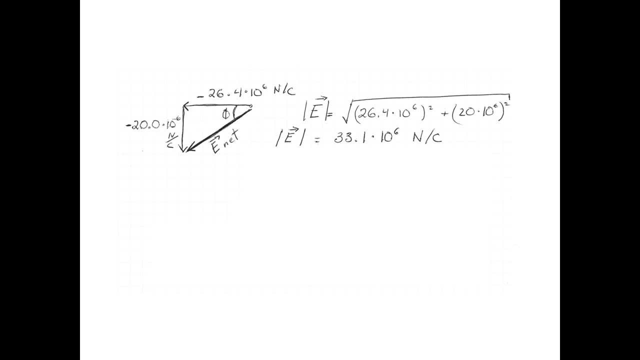 squared plus 20 times 10 to the power of 6 squared, and then the magnitude of my net electric field is 33.1, 10 to the power of 6 newtons per coulomb. The direction is going to be a little bit trickier. 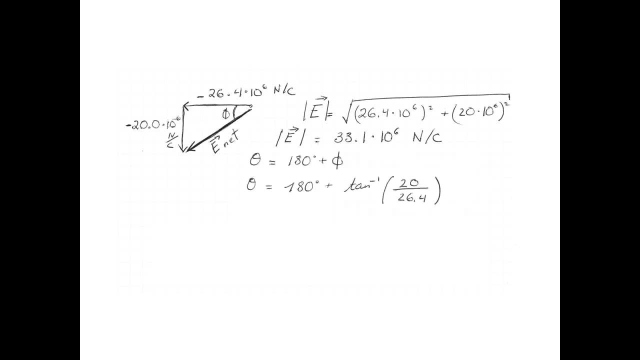 The direction of the vector is 180 degrees plus the angle phi on my picture. That's because you see the vector is to the left and down, so it's in the third quadrant. So 180 degrees plus the inverse tan of 20 divided by 26.4 is 217 degrees And that makes the answer. 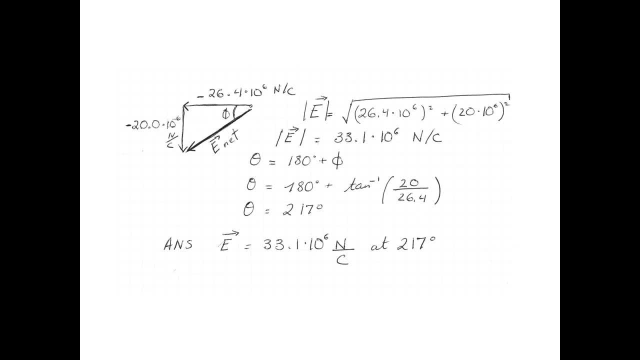 33.1 times 10 to the power of 6 newtons per coulomb at 217 degrees. But wait, Here's a fun extra question. What if we want to multiply the magnitude of the vector by the magnitude of the electric field? What if we want to know the net electric force on a charge q3 placed at point p3?